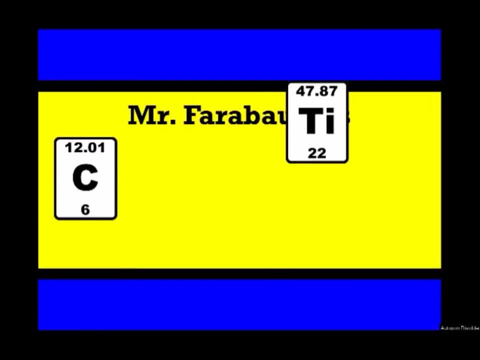 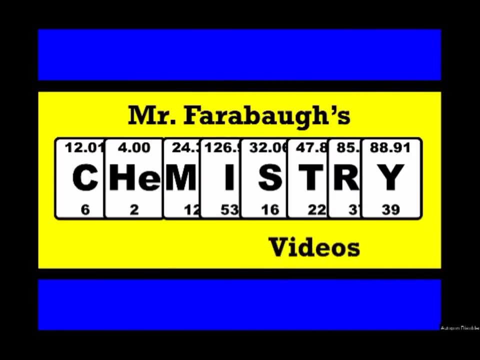 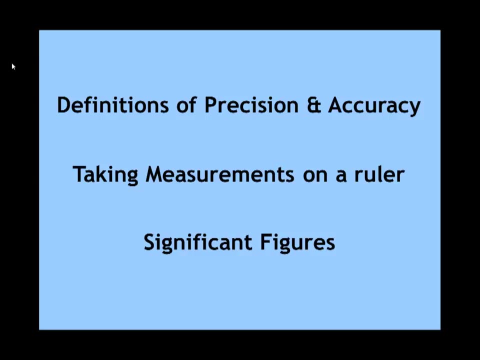 In this video we are going to discuss the definitions of precision and accuracy. I will show you examples of the difference between precision and accuracy. We'll talk about taking measurements on a ruler and how you must add an estimated digit to the end of every measurement. 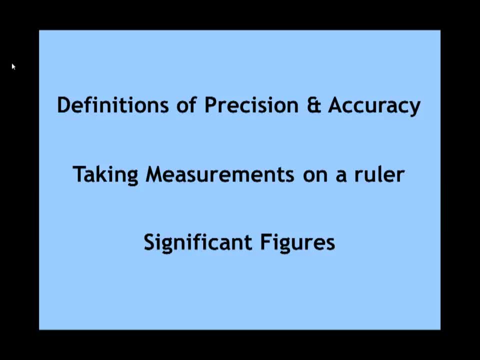 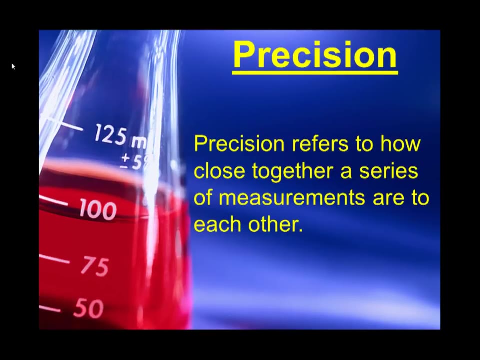 And then we'll also discuss significant figures, or, as I typically call them, sig figs. What exactly are significant figures, and how can you calculate the number of sig figs in a measurement? Okay, let's get started. Definition of precision: Precision refers to how close together a series 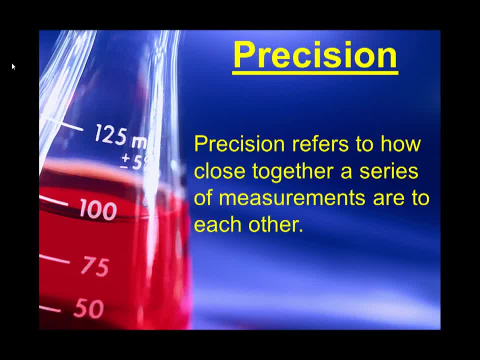 of measurements are to each other. So that means that if you have several measurements and they are all very similar to each other, then that set of measurements is precise. Accuracy refers to how close a measured value is to an accepted value. That means that when the measurement agrees with 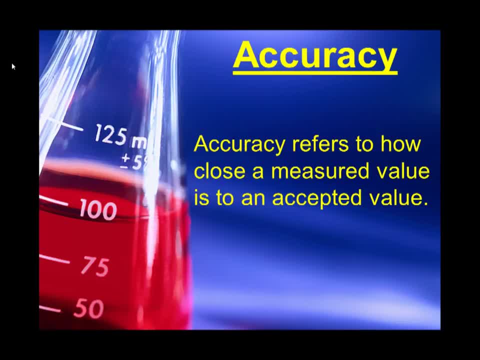 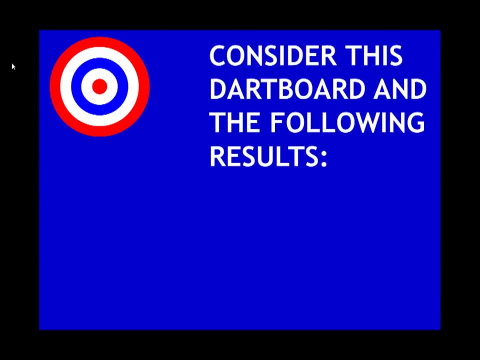 the correct answer or the accepted value, then that particular measurement is accurate. So here are some examples: If a dartboard represents a target and the bullseye would be an accurate measurement, that dart, as well as these next three, did not hit the bullseye, so these are not. 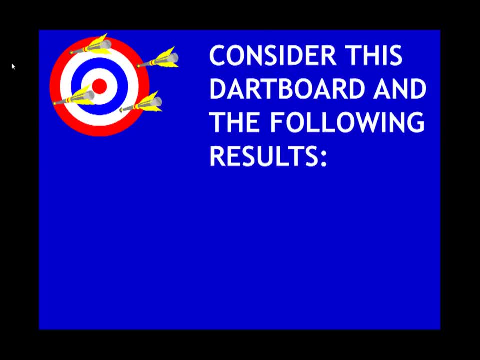 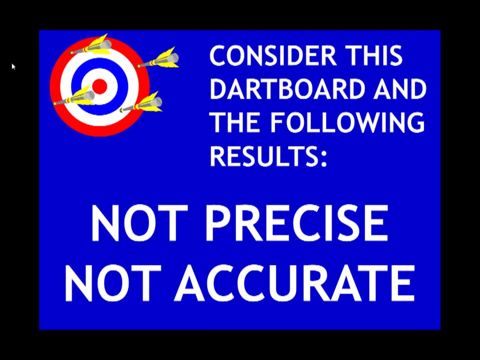 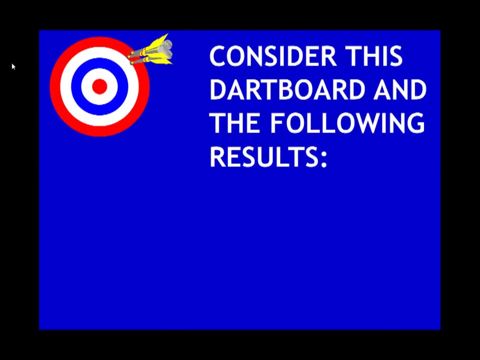 accurate And because they are so spread out, they're not close together. these measurements are not precise. So not accurate and not precise. Now we consider that these darts, while they are not accurate because they're not hitting the bullseye, they are close to each other, These measurements. 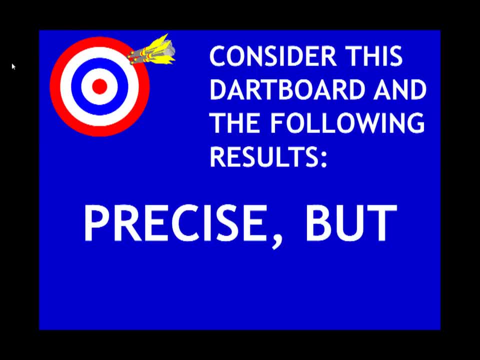 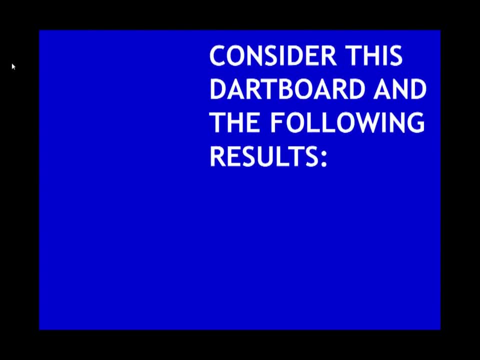 agree with each other. So they are precise because they are close to each other, but again, they are not accurate because they did not hit the bullseye. And finally, in this scenario, the darts are close together and they are on target. 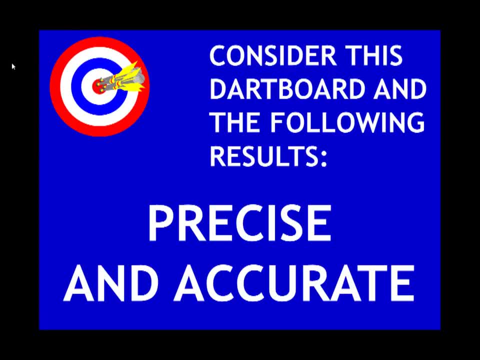 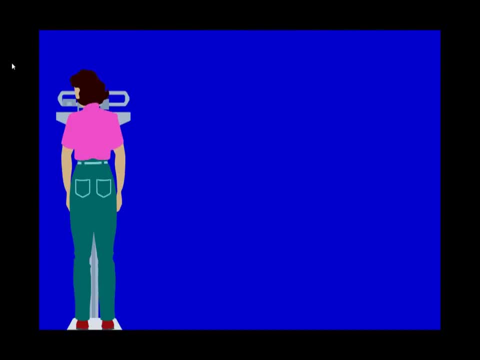 They are on the bullseye, so they are both precise and accurate. Well, now that you understand the difference between precision and accuracy, let's see an example with some numbers. A woman gets on the scale and she wants to decide if the scale is an accurate. 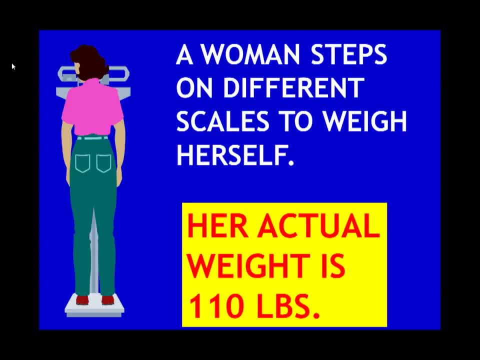 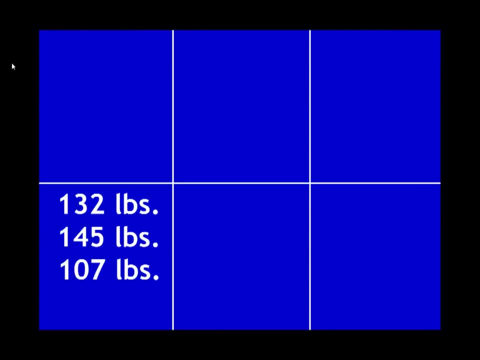 scale. so she decides to weight herself on different scales and her actual weight is one hundred-and-ten 110 pounds. So on the first scale, as you can see from these four measurements, these numbers are not close together and they are not except made. one-oh-seven is sort of close they are. 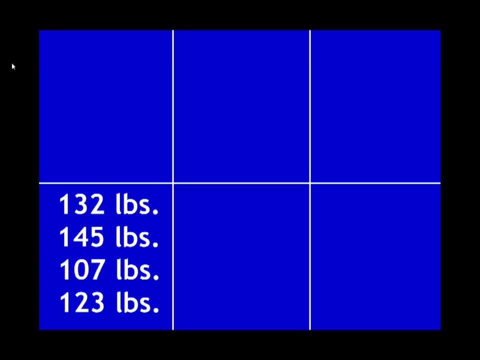 not close to her true weight weight which is 110 pounds. So, like the first dartboard, these measurements are not precise and they are not accurate If another scale gives her the following results when she steps on that same scale four times. while, yes, these numbers are close together: 149 and 150, her. 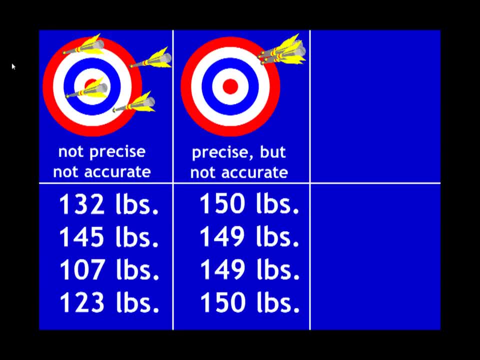 true weight is 110.. So this particular scale is precise because of the consistent reproducible results that she's getting, but it's not accurate. This scale is off by 40 pounds. basically, Finally, if this scale gives her consistent readings that are close together: 109,, 110,. 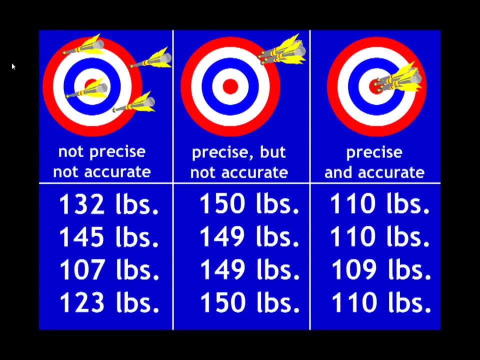 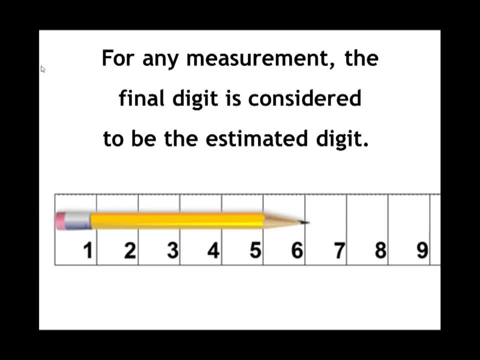 it's both precise and accurate, because the numbers are close together and they are correct. Okay, now we're going to talk about measuring objects on a ruler. As you can see, this is a centimeter ruler. It's not labeled as centimeters, but that's what it is, This pencil. 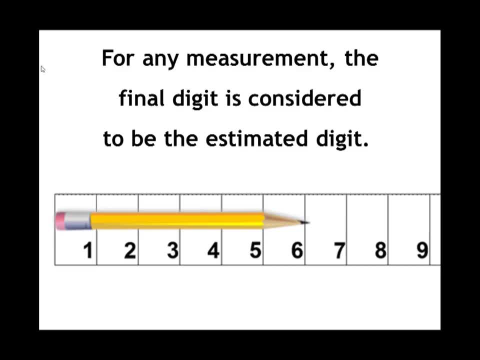 is larger, longer than six centimeters, so we're not able to say it's seven centimeters. It's definitely six point something and that's where the estimated digit comes in. So I, for example, might call this 6.1 centimeters and, as you can see, the one is the final digit and that is. 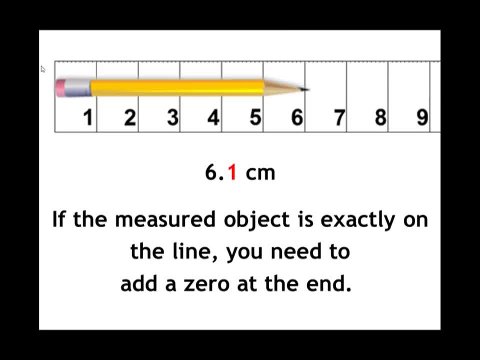 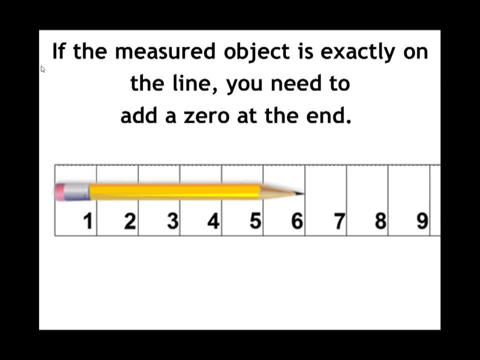 considered to be the estimated digit. Now suppose that we're measuring an object, that's measuring an object where it falls on the line. We still are unable to call this six. We have to say more than that. six point something In this case, because it's exactly on the line. then you 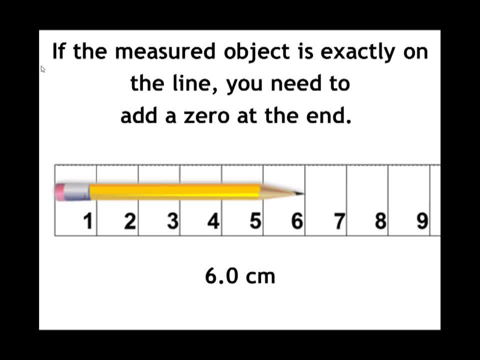 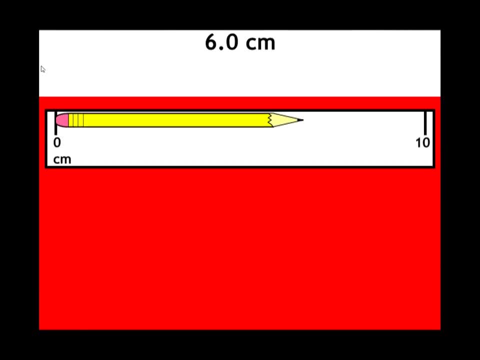 would record this as 6.0, and the zero is at the end of the number and it is the estimated digit, Because it is on the line. you add a zero at the end. Here we have a ruler that doesn't seem to. 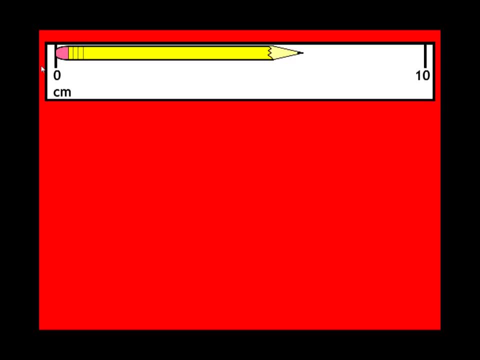 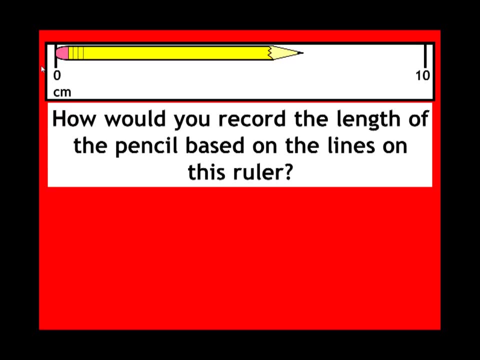 have very many lines on it at all, but it illustrates the point that I would like to make about how you add an estimated digit, In this case to record the length of the pencil based on the lines of the ruler. we know it's going to be somewhere between zero and ten, and that's all we. 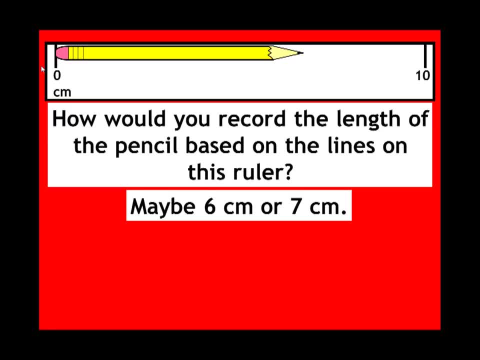 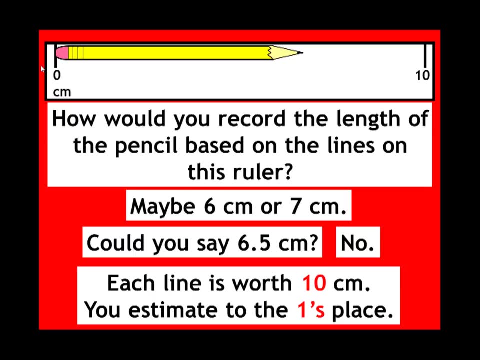 know, Maybe it's six centimeters, maybe it's seven centimeters. Could we say six point five centimeters, And the answer is no. Every line on this particular ruler is worth ten centimeters. so you would estimate to the one's place. 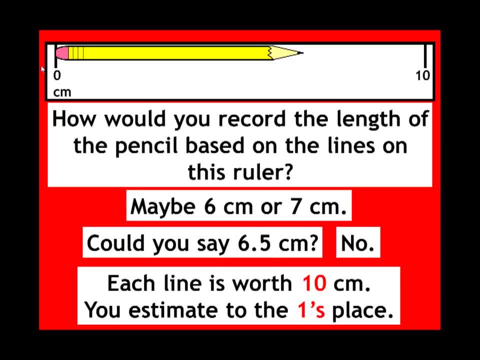 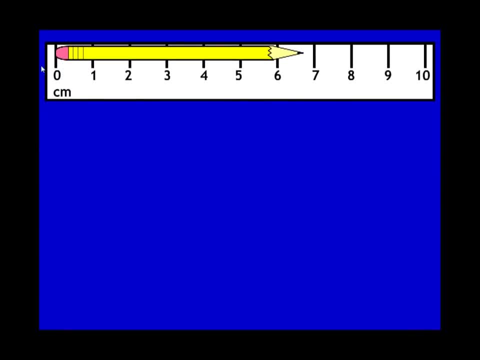 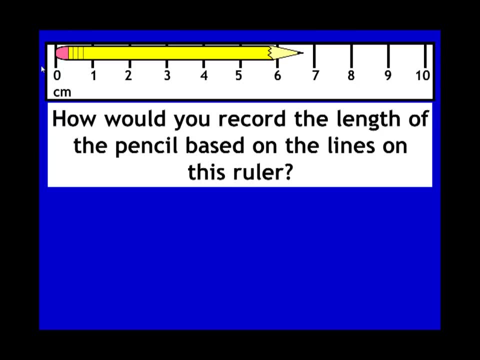 You estimate one power of ten smaller than what the lines are worth. So in this case we could say six, we could say seven, but that's all we could do. Now suppose we have a ruler in which every line that's printed on the ruler is worth one centimeter. We can estimate to the tenth place. so perhaps you might. 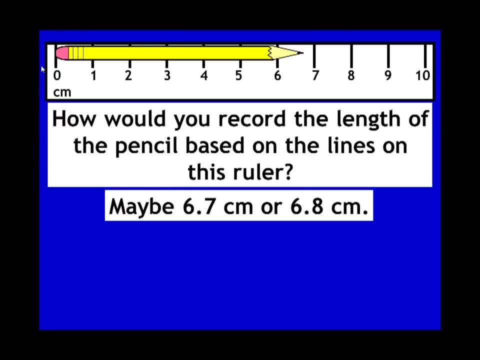 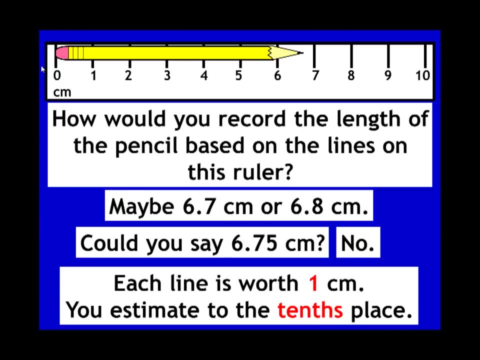 call this six point seven, or perhaps you might call this six point eight. Could we say that this ruler is worth ten centimeters? or could we say that this ruler is worth ten centimeters And the answer is no, Because every line is worth one centimeter. so we can only put the estimated digit one power of ten smaller than what these lines are worth. So six point seven, six point eight, but we could not go out to the hundredth place. We just don't have that level of precision with this ruler. And now, finally, let's go to an even more precise ruler and measure the same object. 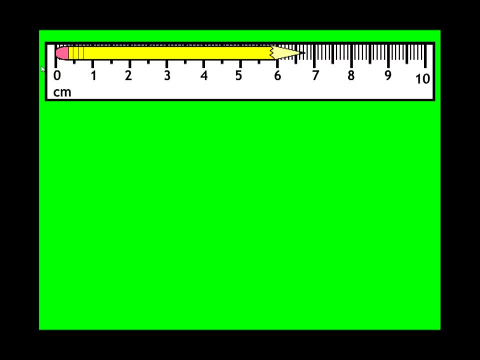 So, as you can tell, this ruler has every line is worth point one, zero point one centimeters. I'm going to give you a close up of expanding what that looks like. So we are now at a point where we can measure somewhere between six point seven and six point eight. 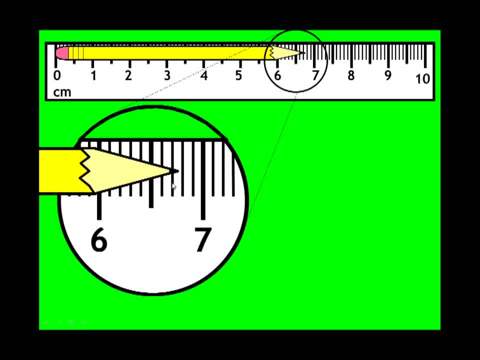 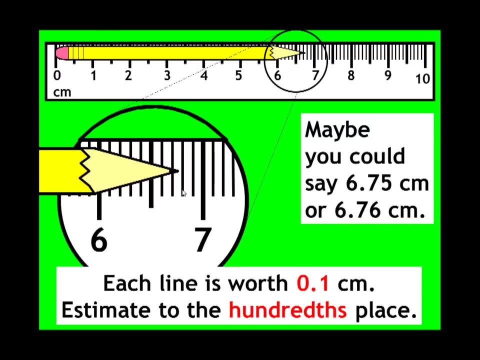 So let's say we think it's roughly about halfway between six point seven and six point eight. You might say that the measurement is six point seven five, or perhaps six point seven six, but the final digit, whatever that number is, is the estimated digit. 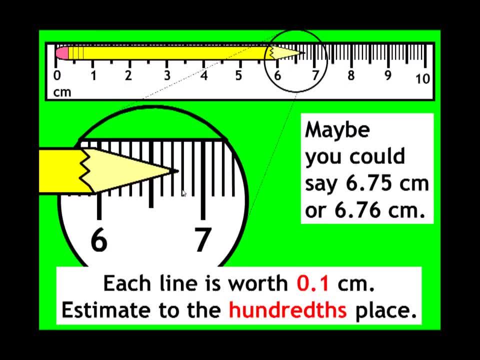 And because every line was worth point one centimeters, the estimated digit was one power of ten smaller than that particular measurement. So we go out to the hundredth place. Okay, now let's consider some examples where the length of the object in some cases is one power of ten. 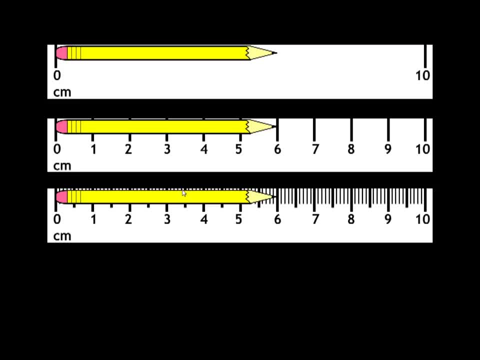 Remember we mentioned that we're going to have to add a zero if the first measurement is just six and we cannot say anything more than that because we are only going to the ones place. But now, with this measurement, we are able to go to the tenth place. 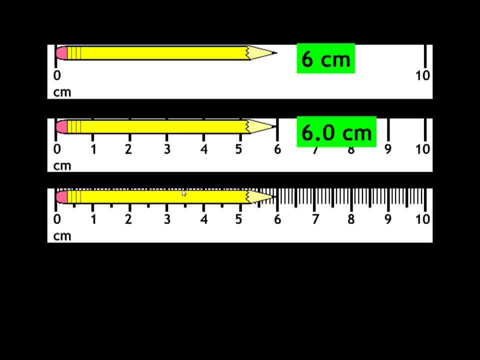 And let's take a moment to think about what that means. I'm saying that six point zero is a more precise measurement than just six. It's a ruler and therefore it does require a different level of precision. So can you guess from this third ruler if we're going now out to the hundredth place with our final digit? this particular pencil on this ruler would be measured as, hopefully, you said: six point zero, zero centimeters. 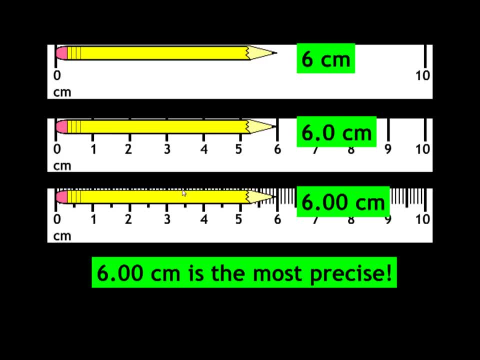 Okay, so that is the most precise of the three measurements. I'm not changing the value. It's still considered six on a calculator, But in a science class six point zero. zero is a different number than six point zero or just six. 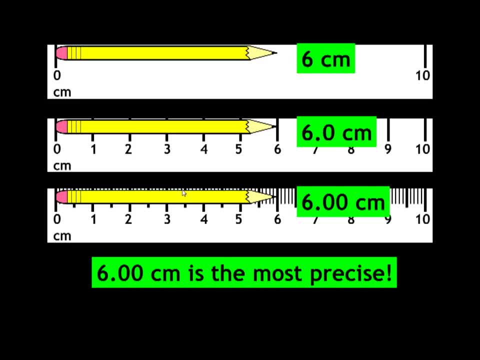 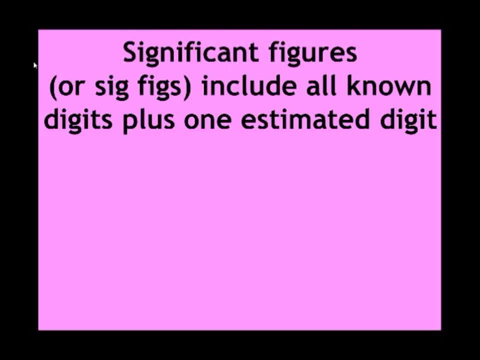 And that leads us to our next discussion, which is we'll be talking about significant figures. Okay, so we're going to talk about significant figures now, or sig figs. In a measurement, the number of sig figs include all of the known digits. 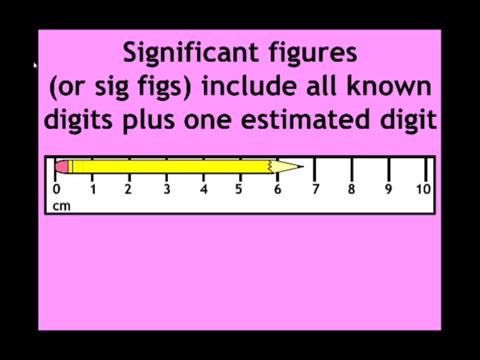 Plus one estimated digit. So in this example the measurement is six point seven. The known digit is a six, Because we estimated that final digit as a seven, that counts as well. It's all significant. so this number would have two significant figures, or two sig figs for short. 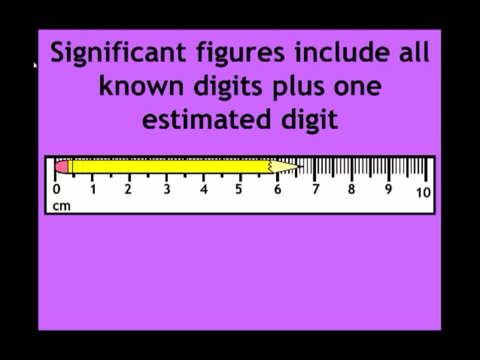 In this example, you can see that we now have a more precise ruler. Take a look at where the final estimated digit should be. Are we going to estimate to the tenth place, Or are we going to estimate to the hundredth place? Hopefully you can see that, because every line that's printed on this ruler is worth one tenth of a centimeter. 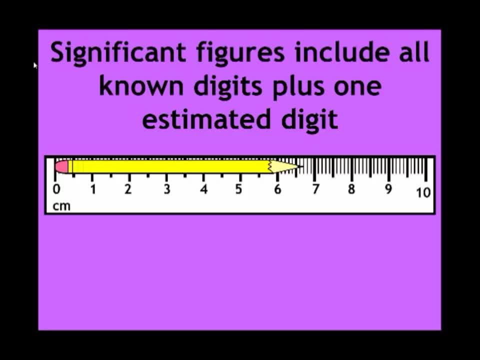 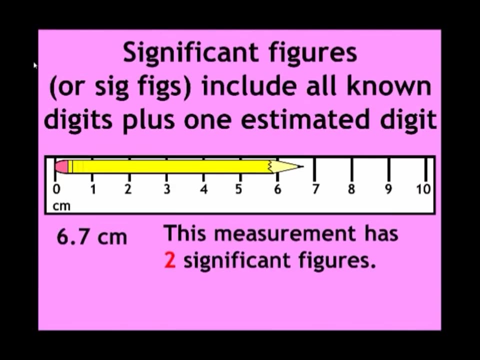 then we will estimate to the hundredth place. So therefore, because it's exactly on the line, it would not just be six point seven. We get to add a zero. So six point seven, zero centimeters. Pay special attention to the fact that I had just shown you six point seven on the previous slide. 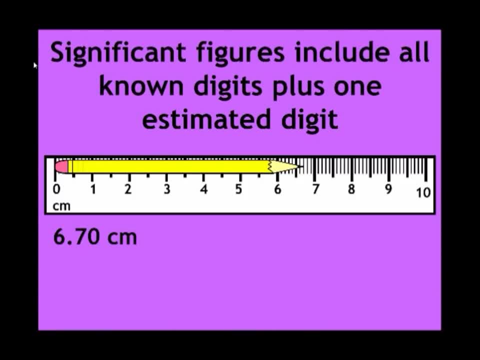 And now I am showing you six point seven zero. So in this chemistry class, six point seven zero is more precise. How many significant figures is a measurement of six point seven zero Three? So this measurement has three significant figures, Not two. 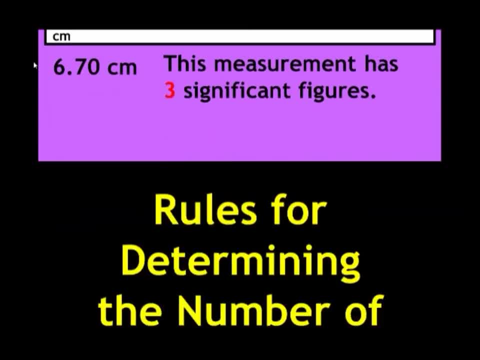 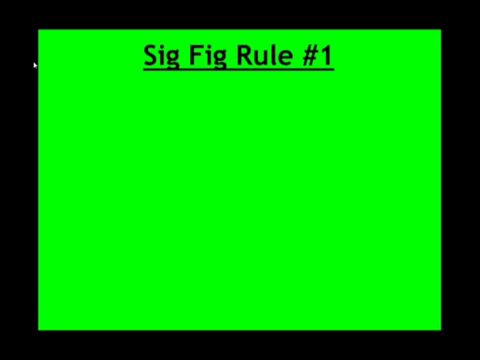 It has three, because we do count that final estimated digit. And now I have to teach you some rules for determining the number of sig figs in any measurement: Sig fig. rule number one: All non-zero numbers are significant. So what does that mean? 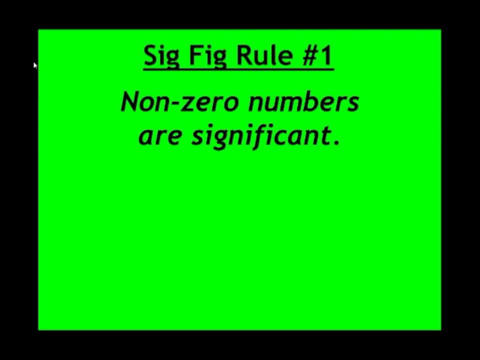 It means any number from one through nine is going to be significant all the time. So here I have a measurement: Seventy two point three grams. There are no zeros, Everything counts. This measurement has three sig figs. Okay, Our next sig fig rule. 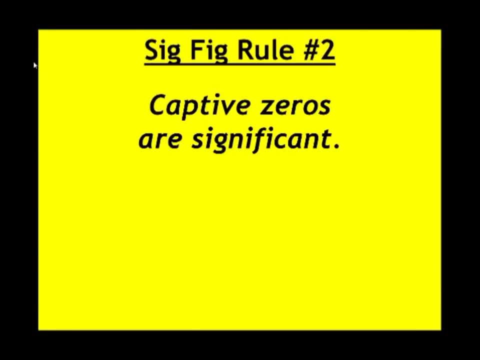 Sig fig rule number two: Captive zeros are significant. So what does that mean? What are captive zeros? A captive zero is a zero that is trapped in between non-zero digits. Here's an example: Eight hundred point four centimeters- The eight, we know that counts. 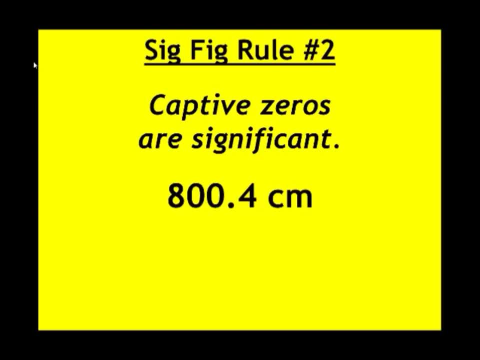 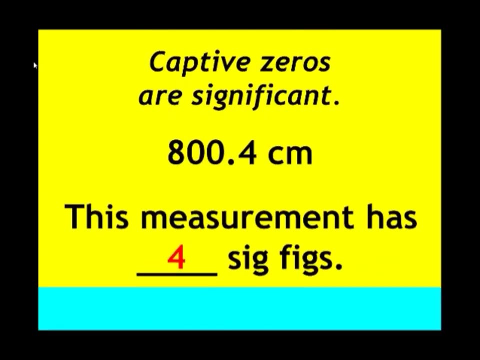 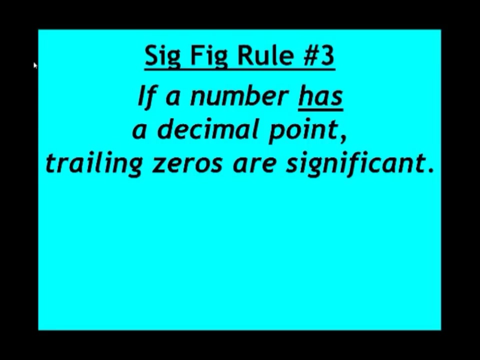 The four. we know that counts, And those two zeros are captive, They are in between. So everything counts in this measurement. This measurement eight hundred point four has four significant figures. Okay, On to sig fig rule number three: If a number has a decimal point, then the trailing zeros, the zeros at the end of the number, are significant. 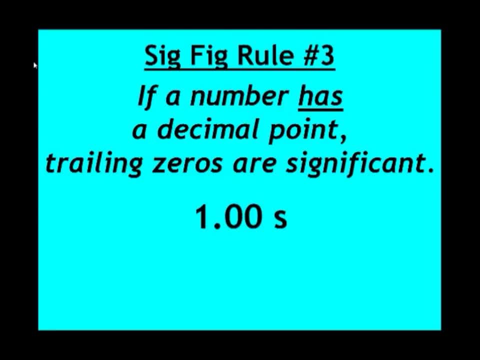 So here is a number: One point zero, zero. It's a measurement One point zero, zero seconds. It has a decimal point. The zeros at the end are significant. So therefore, a measurement of one point zero, zero seconds has three sig figs. 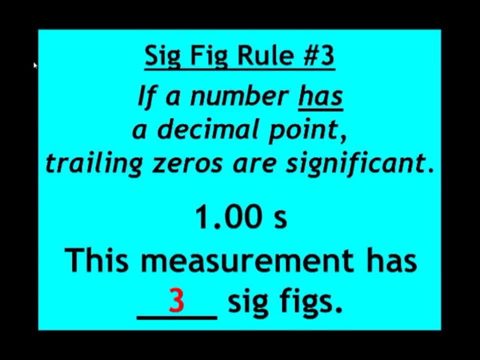 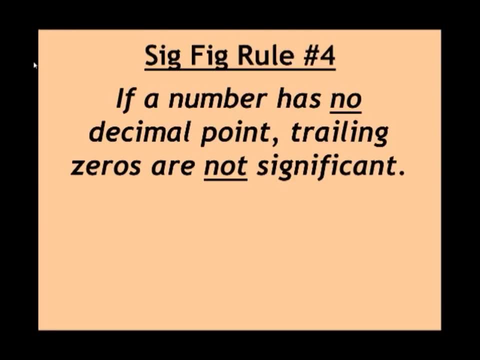 Okay, Moving on to sig fig rule number four, If a number has no decimal point, then the trailing zeros which are at the end of the number do not count. They are not significant. So notice the measurement. One thousand five hundred liters. 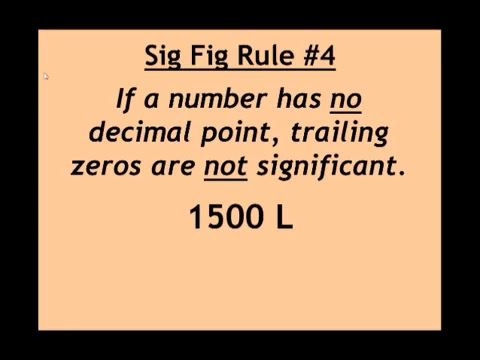 There is not an exact point. There's no decimal at the end of a number, So we have fifteen hundred or one thousand five hundred, but these two zeros are now no longer significant. A measurement of one thousand five hundred liters has two sig figs. 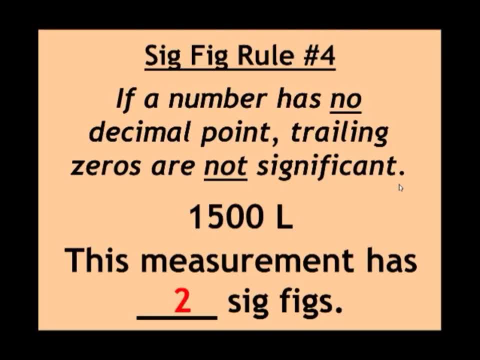 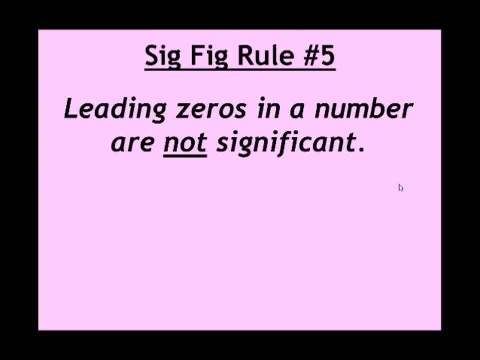 Okay, And our final rule, Sig fig. rule number five: Leading zeros, which are the zeros that occur at the beginning of a number. Typically, this would mean you have a number that is less than one, So leading zeros at the beginning of a number are not significant. 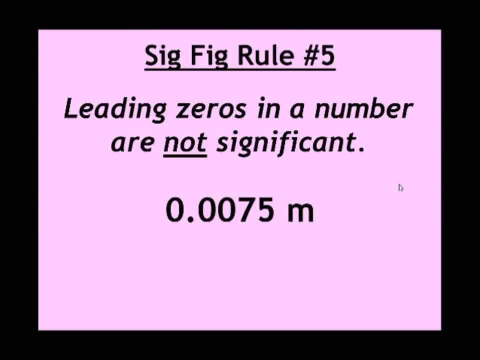 So we have a number that would be zero point zero, zero, seven, five. This measurement has three leading zeros, But according to sig fig rule number five, these are not supposed to count. Therefore, a measurement of zero point zero, zero, seven, five meters has two sig figs. 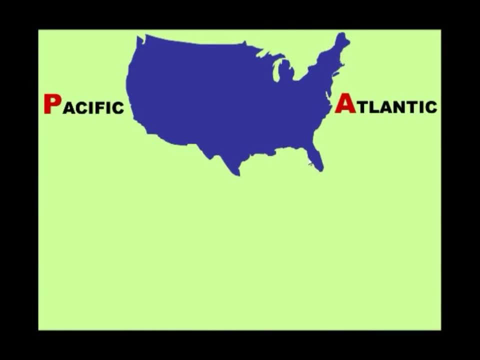 Okay, So now the last thing I would like to show you. if you are confused about all of those rules that you just saw And remember, you are welcome to replay this video as many times as you like, And you can pause the video to take notes. 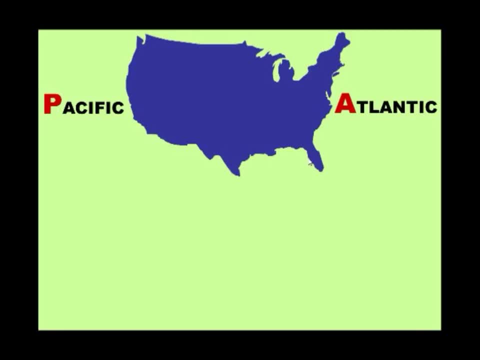 I'm going to give you a little rule, a mnemonic device for remembering the number of sig figs in a measurement, And I call it the Atlantic and Pacific rule. So clearly you can see there is an Atlantic on the right and a Pacific on the left. 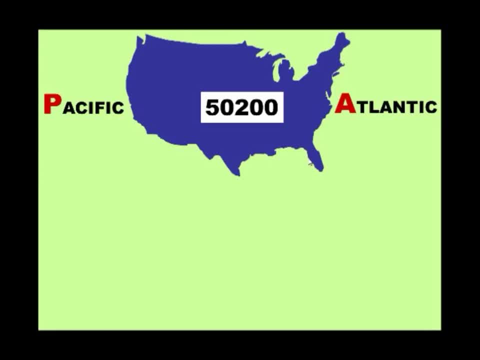 So here is the first application of the Atlantic and Pacific rule. A number is given to you And we will assume that is a measurement, even though there is no unit. Let's just pretend that there is a unit: Fifty thousand two hundred something. 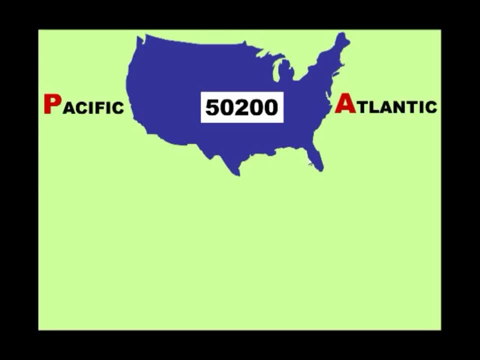 That could be seconds, meters, grams, It doesn't matter. I'm focusing on the number. If a decimal is absent- A for absent, A for Atlantic- You will start counting from the Atlantic side of the number, That is, from the right. 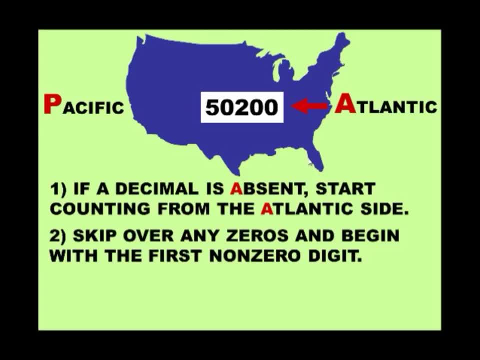 Skip over any zeros that you encounter on that side, So I'm going to just cross them out And begin with the first non-zero digit. So the first number I come to that is not a zero happens to be a two. Then continue counting every single digit, no matter what it is. 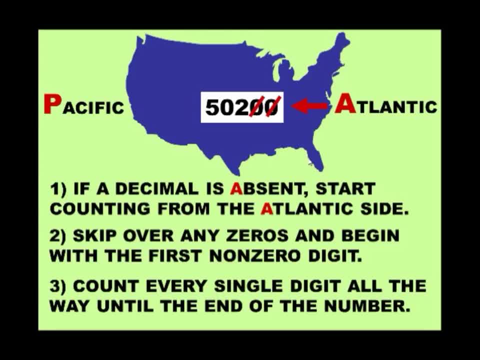 Zero through nine. Every single digit is now considered significant, all the way until you get to the end of the number. This measurement of fifty thousand two hundred has three sig figs, And this is according to the Atlantic rule. You use the Atlantic rule when a decimal is absent. 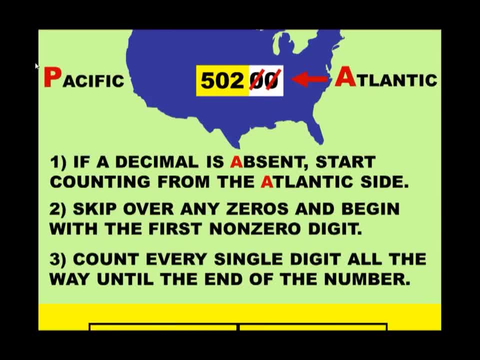 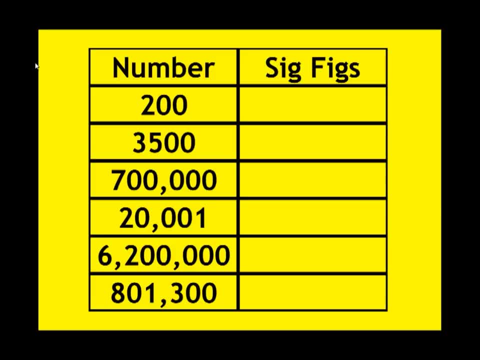 Let's go ahead and practice examples of the Atlantic rule. So you have to forgive me for not showing you units. All we have are numbers. We have to assume that these were all measurements. Two hundred. It could be grams or meters, That doesn't matter. 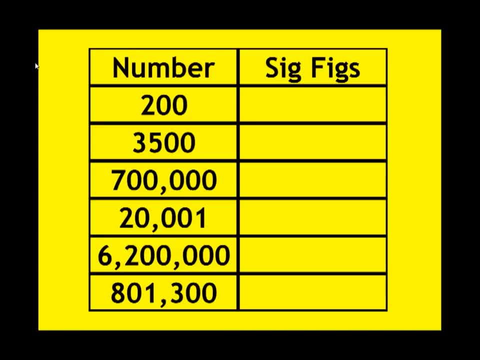 I'm just kind of focusing on the number right now. Every single one of these six numbers is going to obey the Atlantic rule, Because in every single number a decimal is absent. So A for absent, A for Atlantic, If we count from the right side of the number, 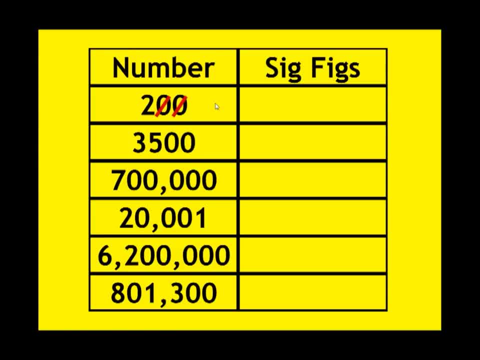 And I'm going to go ahead and just skip over any of the zeros that are on that particular side of the number. Whatever we have left from that point forward, from the end of the number, is going to be the number of sig figs. So two hundred has one sig fig. 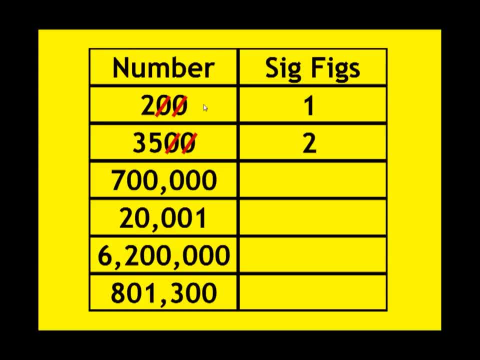 Three thousand five hundred has two sig figs. Seven hundred thousand has only one sig fig. Now in the next example it's twenty thousand and one. There must be a reason for twenty thousand and one, because it would be counted to the ones place. 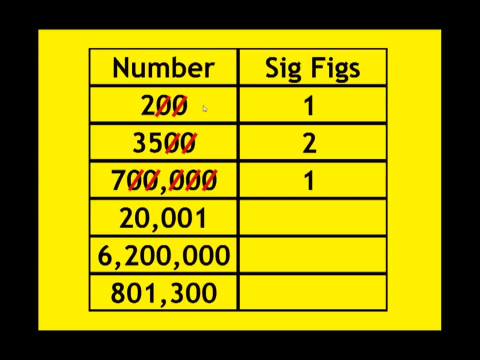 For whatever reason, The first number we come to on the Atlantic Ocean side is a one. So therefore, since a one is significant, everything else counts. You may remember that that's the sig fig rule number two: Captive zeros are significant. Then we come to a number which is really large. 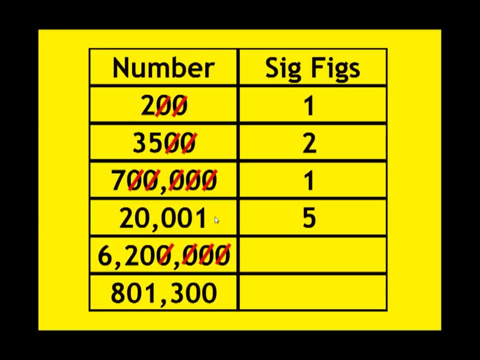 Six million two hundred thousand. If we skip over all of the trailing zeros because the decimal is absent, We get only two sig figs And then finally eight hundred and one thousand three hundred. The decimal is absent, Atlantic Ocean side. Once we get to the three. 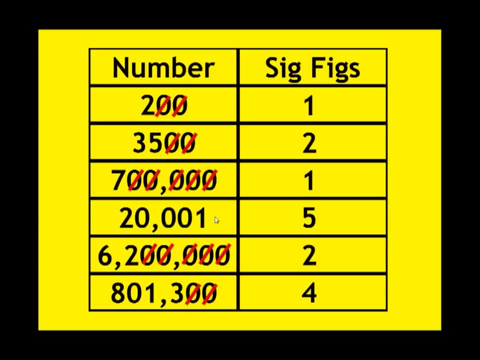 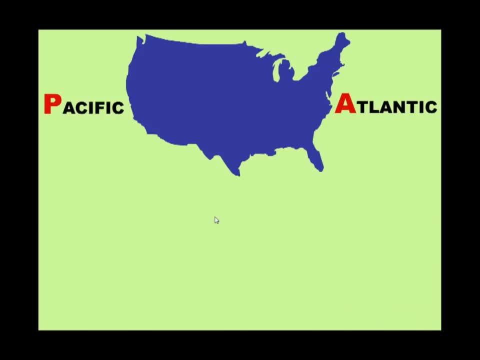 Everything counts. So this number has a total of four sig figs. So if the Atlantic rule applies when a decimal is absent, We apply the Pacific rule when a decimal is present. Now we start counting from the Pacific Ocean or the right side. 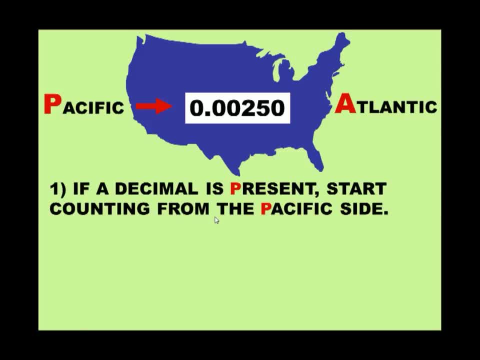 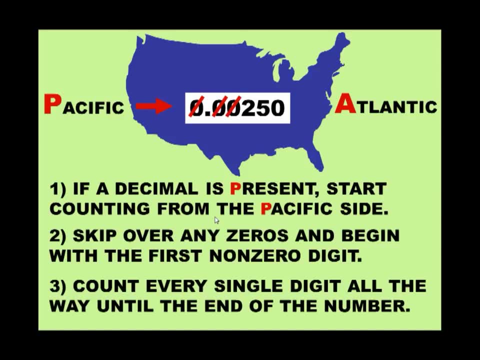 Excuse me. So we count from the Pacific Ocean side, or the left side of the number, Skip over any zeros, as we did before, And once you come to a non-zero digit, Then you count every single digit all the way until you get to the end of the number. 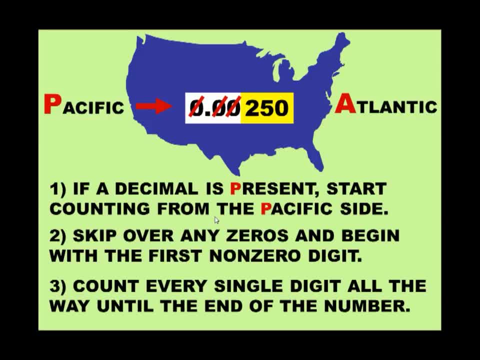 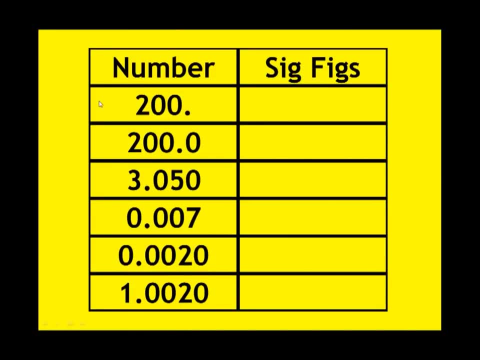 So this particular measurement of zero point, zero, zero, two, five zero Contains three sig figs according to the Pacific rule. And now it's time to practice the Pacific rule. So all six of these measurements Contain a decimal point. We'll start counting from the Pacific Ocean or the left side of the number. 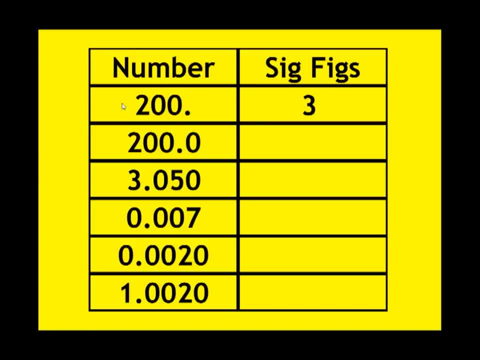 Two hundred with a decimal point at the end Implies that you have confidence Out to the ones place. That measurement has three sig figs. Two hundred point zero Again, because you're counting from the Pacific Ocean side, The first number you come to is a two. 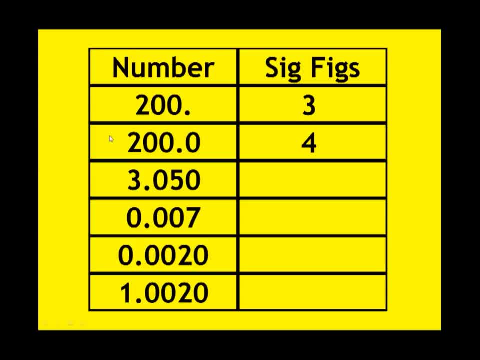 And from that point forward Everything counts. So four sig figs For that measurement. Similarly, Three is the first number we come to on the Pacific Ocean side, So everything counts: Four sig figs. But now what do we do with this next measurement?